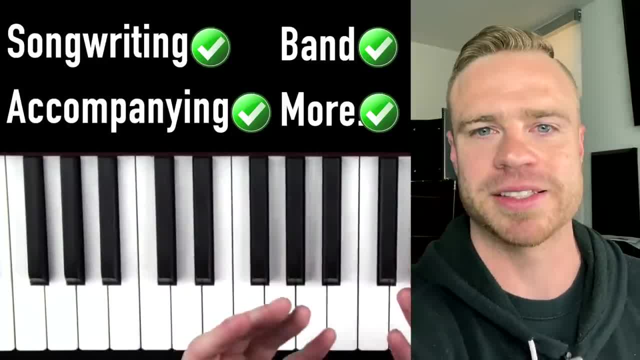 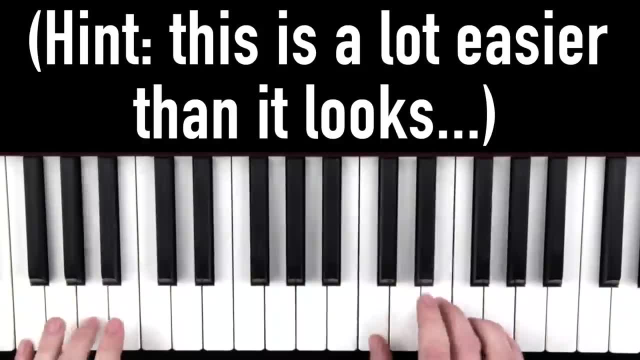 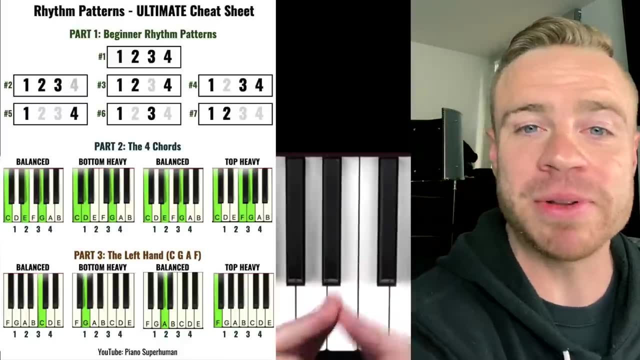 And at the end of the lesson you'll be able to play stuff that sounds something like this: I'm going to break this down with the cheat sheet to make it so easy. a complete beginner who's never touched a piano in their life could learn it. 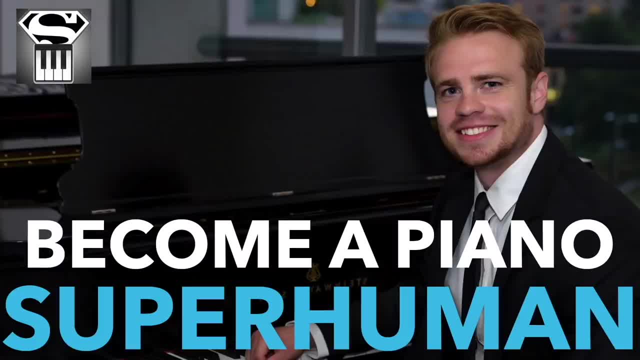 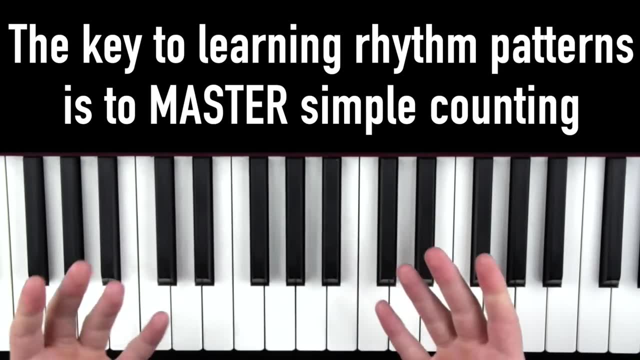 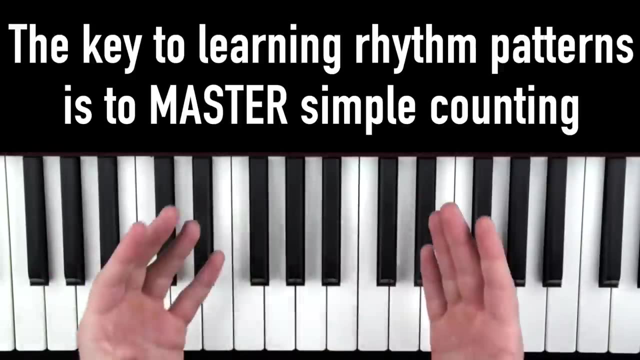 All right, I'm excited and ready to go. Let's get started. All right, so the key to learning rhythm patterns is actually just to get really good- Good at simple counting. Once you master simple counting, even advanced rhythms are going to be a piece of cake. 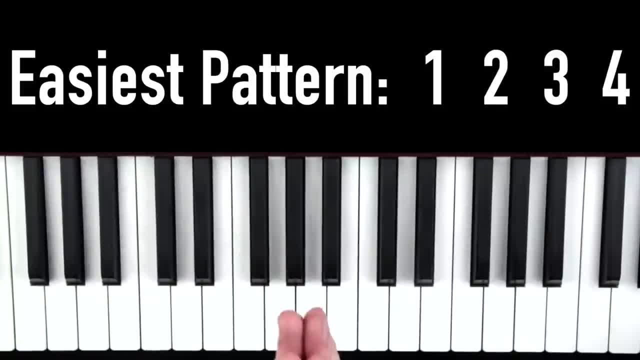 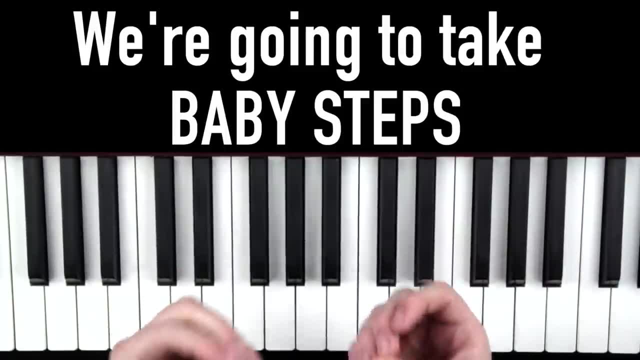 All right. so the simplest rhythm is simply 1,, 2,, 3,, 4.. All right, and we're going to take absolute baby steps to make sure 100% you get this, even if you are a complete beginner, so that you don't get frustrated, okay. 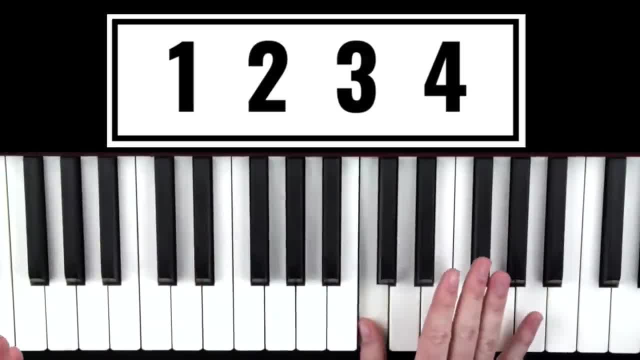 So what I want you to do is put your right thumb on C and count as you play, And just count 1, 2,, 3, 4.. It's going to sound like this: 1, 2. 3.. 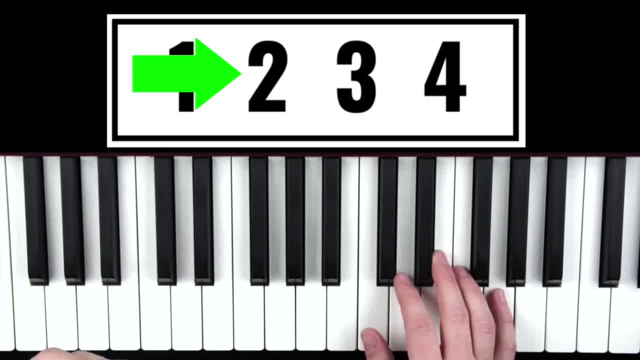 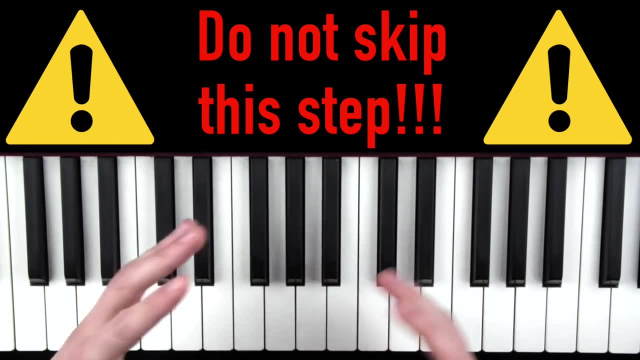 4., 1., 2., 3., 4. Right, don't say 5.. There is no 5, right, Just 1,, 2,, 3,, 4.. Now I know this might sound super, super easy, but do not skip this step, okay. 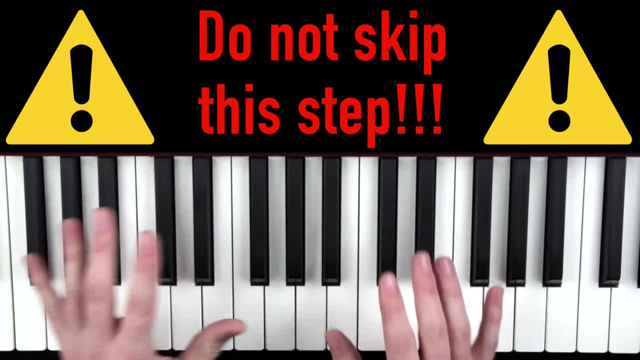 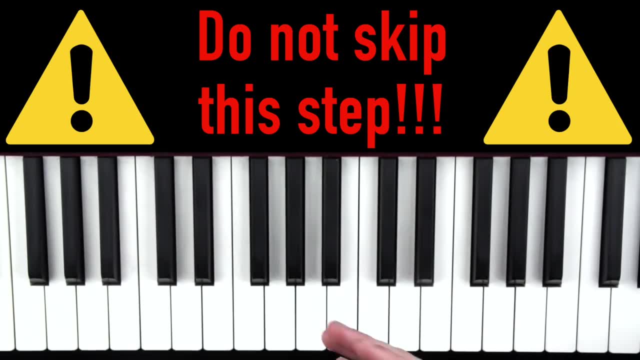 We have to start integrating counting into your brain even at the simplest step, so that when we start adding more advanced rhythms, the counting becomes automatic and it's locked into your brain. So make sure that you're actually counting While you're playing. if you can count out loud, even better. 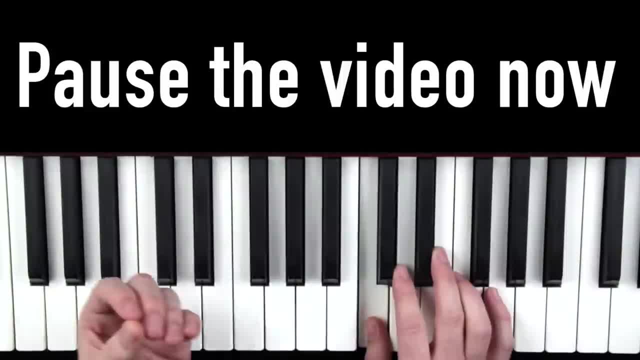 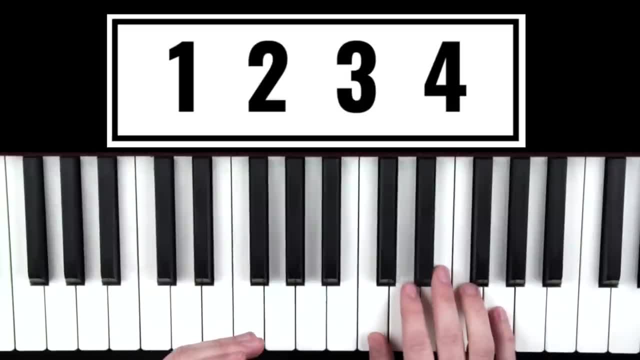 So pause the video now and work on your 1,, 2,, 3, 4.. All right. next step is we're simply going to add an E with our middle finger, So we have C and E, And guess what? We're going to do the exact same thing with these two notes. 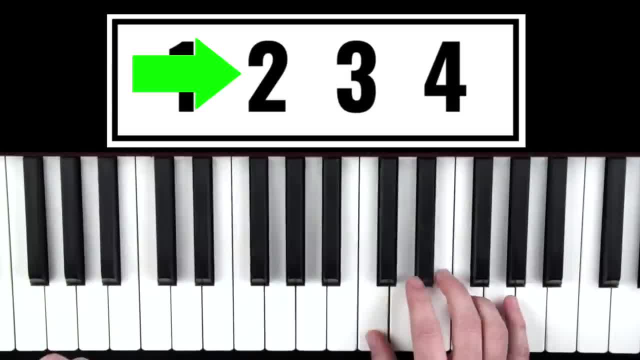 So we're just going to count 1,, 2, 3, 4.. 1,, 2,, 3, 4.. Now make sure you're actually counting. okay, Don't get lazy here. Pause the video and work on your C and E. 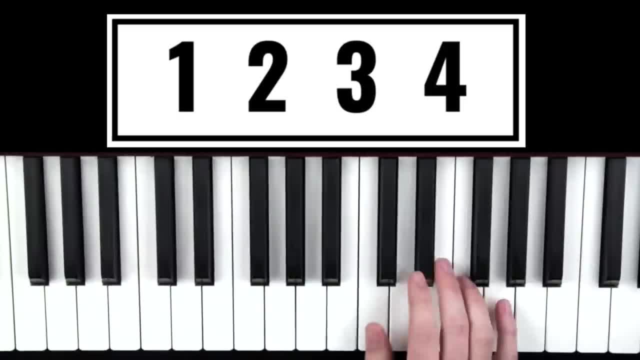 All right. finally, we're going to add the top note to this pattern, to complete the C chord by adding the G note on top with your pinky. So we have C, E and G, And guess what? We're going to do the exact same thing, okay. 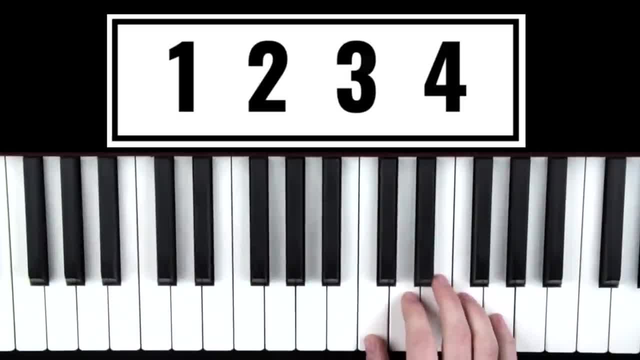 Let's drill this: 1, 2,, 3, 4 with the G on top. It's going to sound like this: 1, 2, 3, 4.. 1,, 2,, 3, 4.. 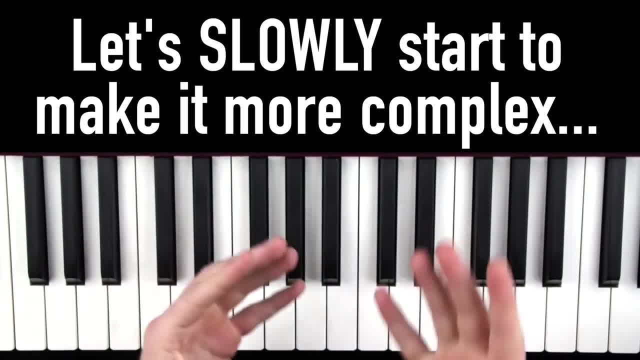 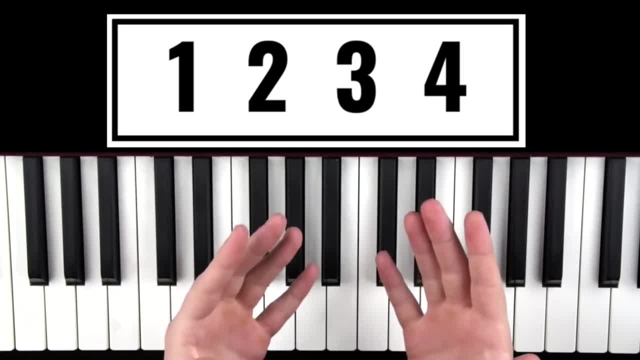 All right, pause the video now and work on it. All right, so now that our counting is starting to feel automatic, let's slowly and gradually start to complicate things. All right, so all we have to do to make a complex rhythm out of 1,, 2,, 3, 4 is remove any of the numbers 1,, 2,, 3, or 4.. 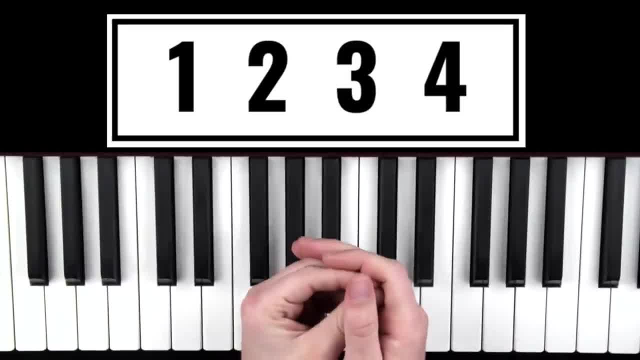 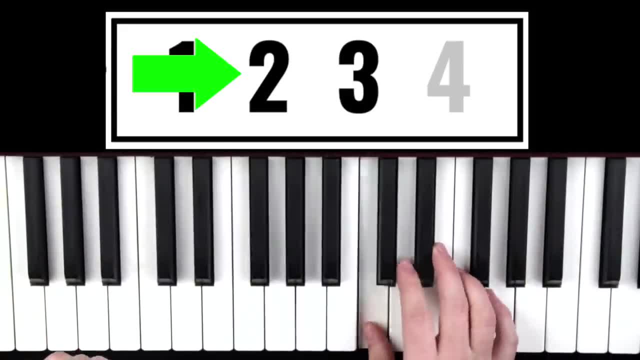 All right. so first let's remove the number 4, right, And let's just go back to just playing our thumb, and it's going to sound like this: 1, 2, 3, 4.. 1,, 2, 3, 4.. 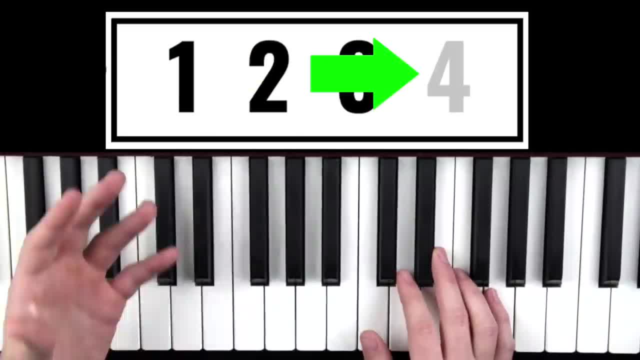 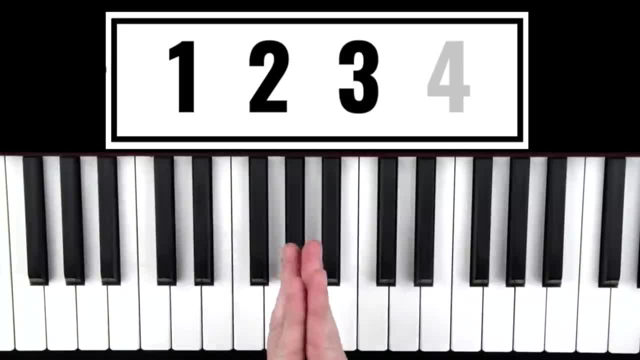 1, 2,, 3, 4.. Now it's really important to count the number 4, even though you're not actually playing it. When we get onto harder rhythms, you need to count to keep your brain locked into the rhythm, even when you're not playing a note on that beat. 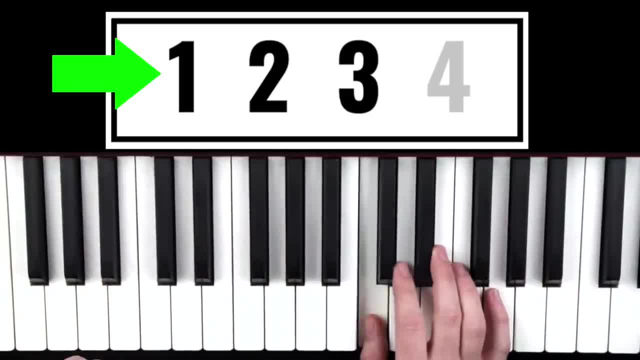 So once again, with the thumb, it sounds like this: 1, 2,, 3, 4.. 1,, 2,, 3, 4.. And once you get that good, just like before, we're going to add our middle finger. 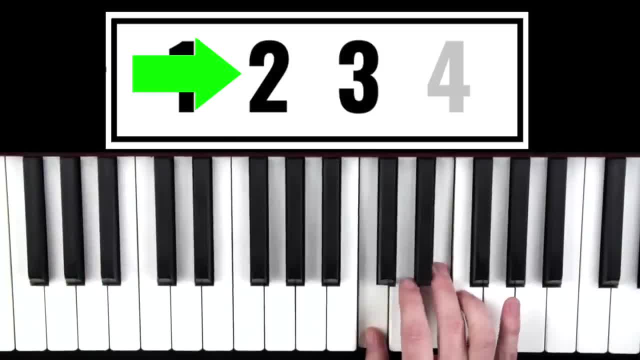 Same thing, right: 1, 2,, 3, 4.. 1,, 2,, 3,, 4.. And then, of course, once that's good, we're going to add the pinky on top. 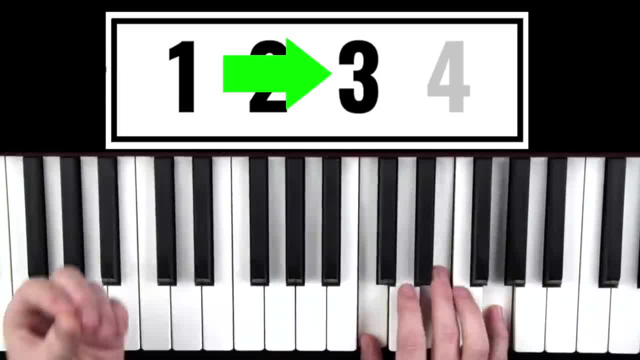 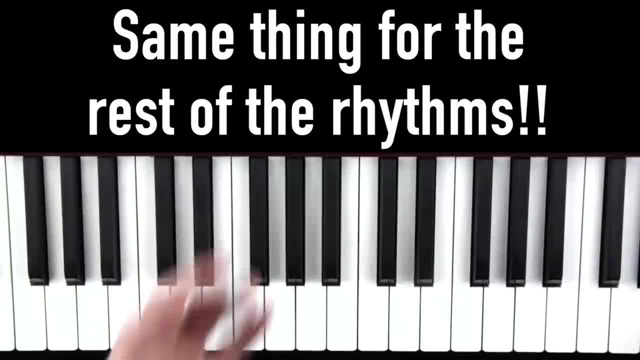 Now for the rest of the rhythms we're going to cover. we're going to do the exact same process. Okay, step 1, play it just with your thumb. Step 2, play it with your thumb and your middle finger. 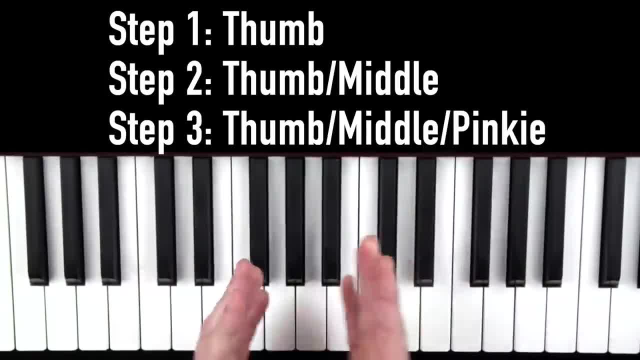 And step 3, play it with your thumb, middle and pinky And the whole time counting while you play. Now, if you're a beginner, it's very important that you follow this process to drill in counting correctly and solidly into your brain. 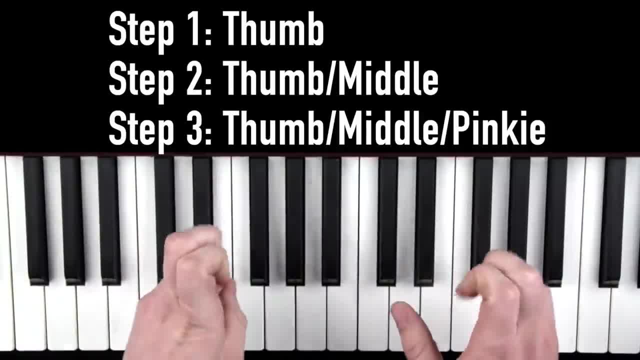 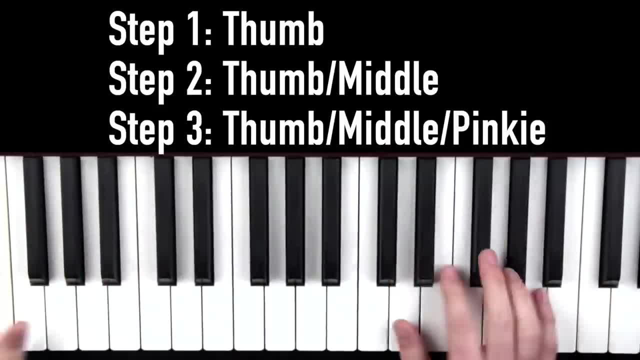 You know it's crazy to me how many YouTube videos I see out there that are, you know, quote unquote for beginners And they have like one-minute instruction And then they're like, alright, just play this rhythm over a 1,, 5,, 6 chord progression. 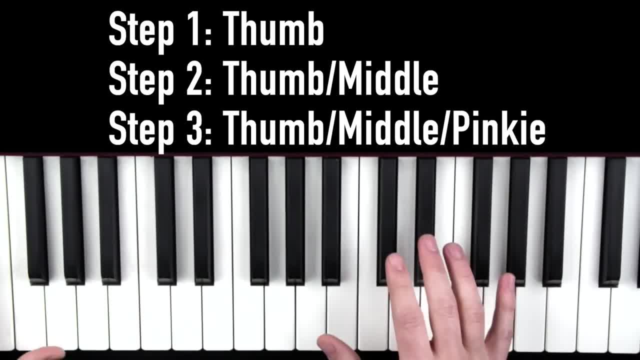 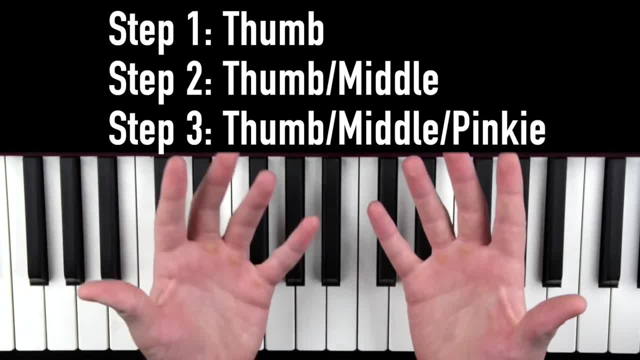 And I'm like what You just added: chord inversions, left-hand octaves and rhythms all at the same time And they just plow on to the next thing. If I was a beginner I'd be like yo, what are you talking about, right? 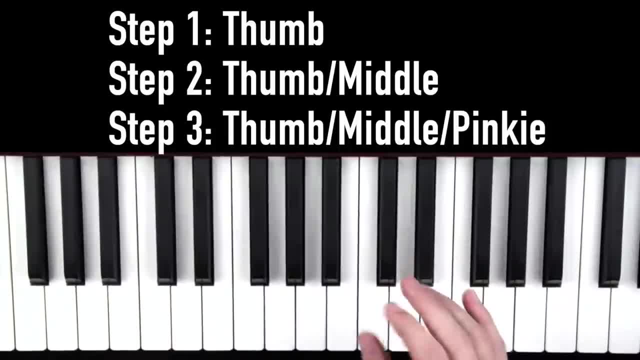 So it's very important that you follow these three steps of thumb, then thumb middle, then thumb middle, pinky. I'm really breaking down everything into tiny, tiny steps, Tiny baby steps for you, to make sure you don't get frustrated. 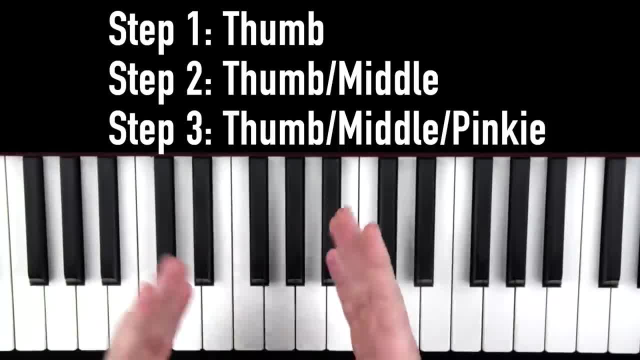 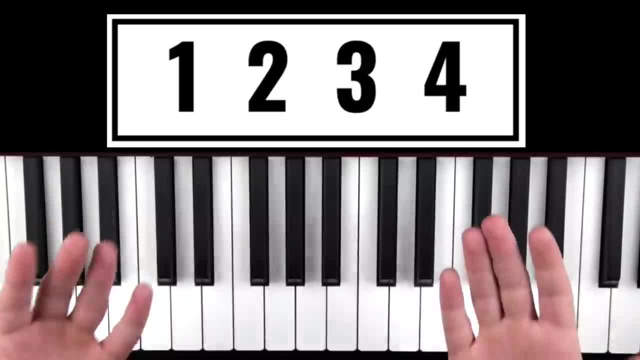 And then make sure that you're counting out loud if possible, and playing at the same time. Alright, so let's try another rhythm pattern Now. this time, instead of removing the number 4,, let's remove the number 3.. 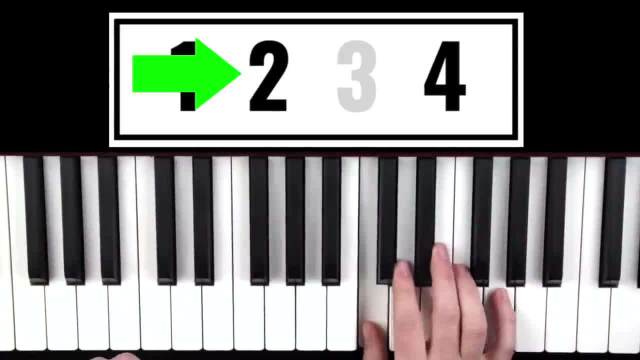 So now it sounds like this: 1,, 2,, 3, 4.. 1,, 2,, 3,, 4.. And do the same thing. right, then we add our middle finger: 1,, 2,, 3,, 4.. 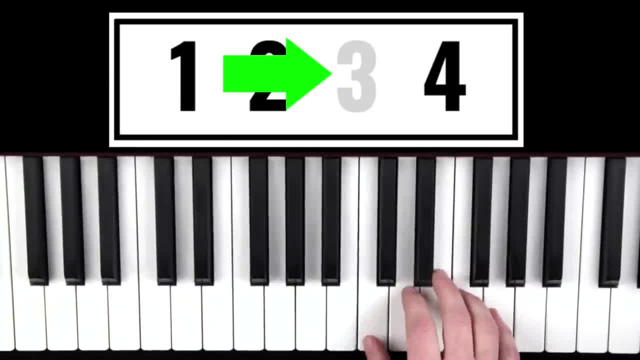 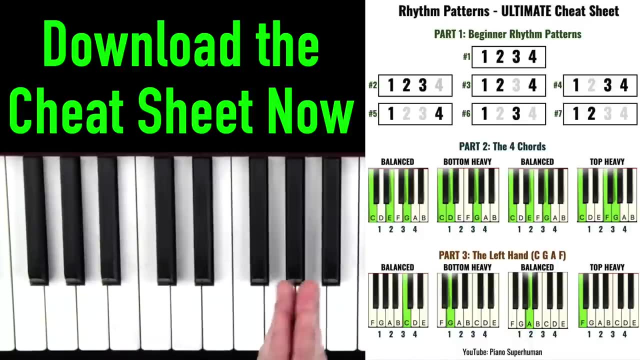 1,, 2,, 3,, 4.. And finally, the pinky: 1,, 2,, 3, 4.. 1,, 2,, 3, 4.. Alright, before we add the next rhythm pattern, this would be a great time to download the cheat sheet. 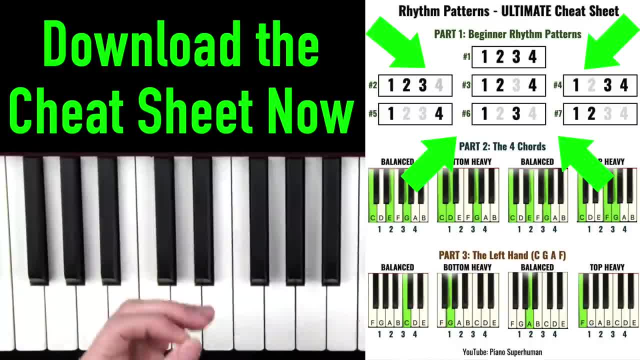 This way you don't have to remember all of these rhythms. It'll be right there on the cheat sheet for you, And it has a bunch of stuff we're going to use later in this lesson anyway as well. So click the link here in the description. 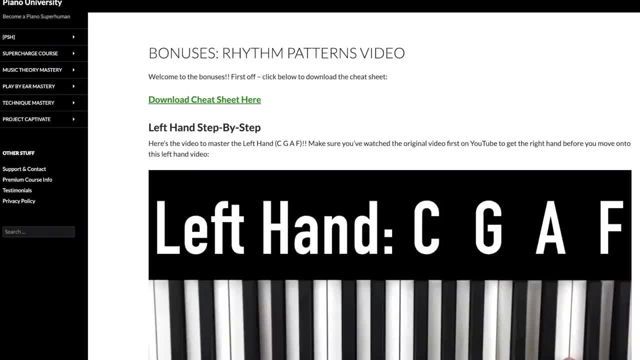 You'll go to this page, enter your name and your email and you'll go to the bonuses page, Then click here to download the cheat sheet. Alright, so go download the cheat sheet now and I'll see you back here soon. 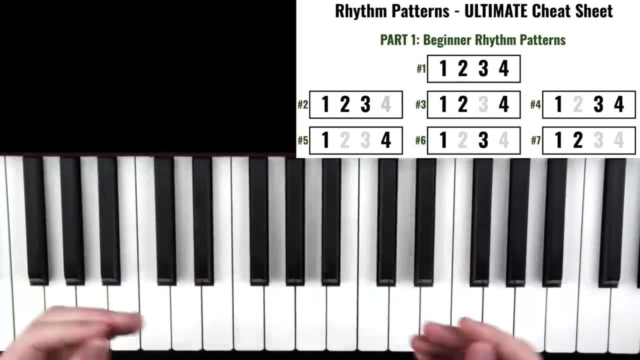 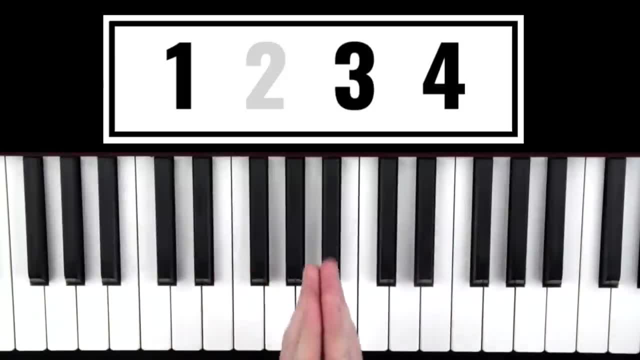 Alright, so go to your cheat sheet under the beginner rhythm patterns And you'll notice we already practiced 1,, 2, and 3.. So now, if we find rhythm number 4,, as you can see, for this one we just remove the number 2.. 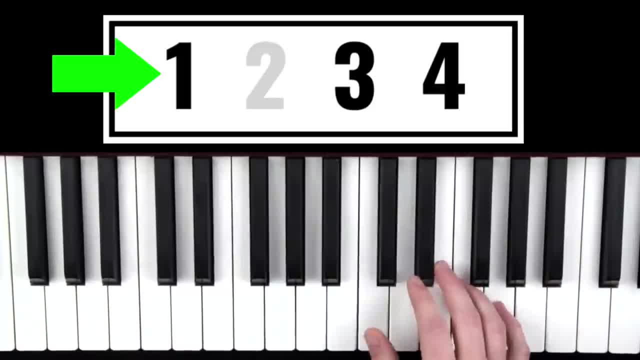 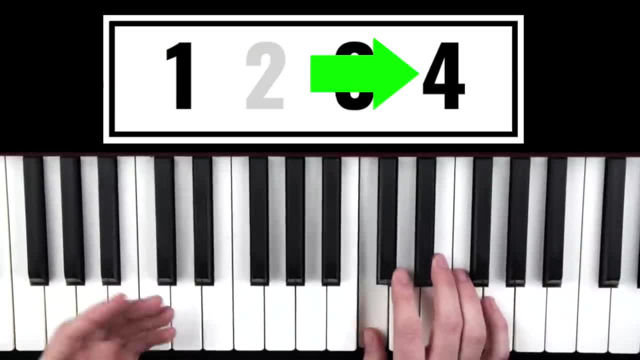 So, as you play it, it simply goes like this: 1,, 2,, 3, 4.. 1,, 2,, 3,, 4.. And of course, you would practice that rhythm pattern again with your thumb and middle finger. 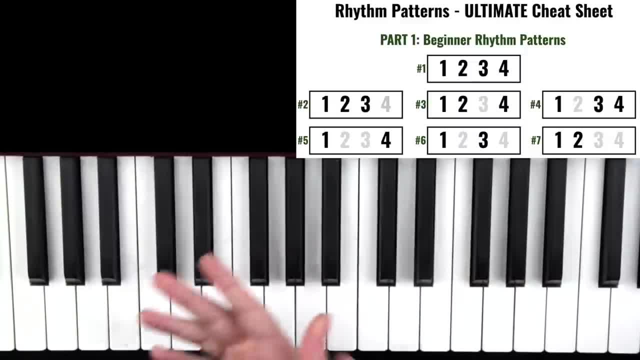 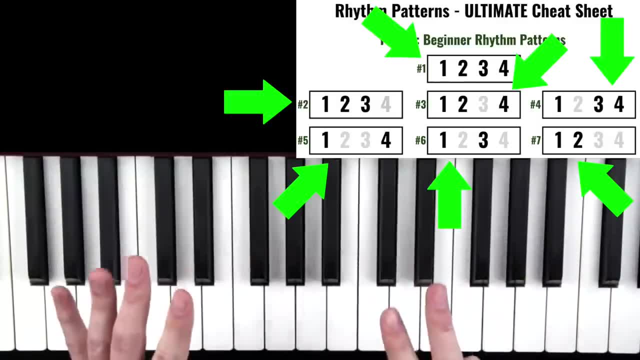 And then, of course, adding the pinky: Alright, so now that you get the process of learning these rhythm patterns, you can explore the other core beginner rhythm patterns. on the cheat sheet There are seven of them And you don't need me to learn them, right. 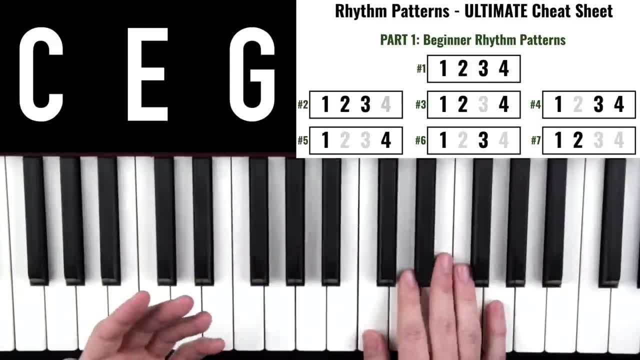 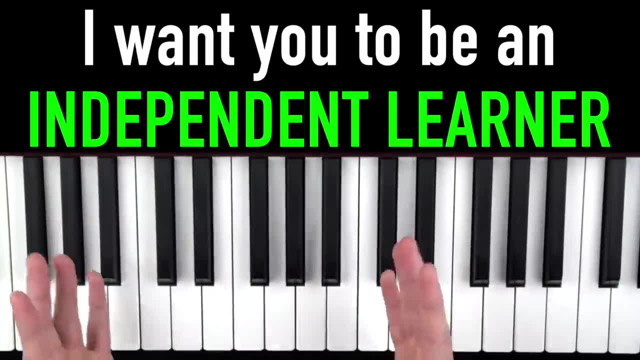 Just follow the steps that we've been doing for the other rhythm patterns. We started with thumb, then thumb middle, then thumb middle- pinky. I want to make you an independent learner where I don't just tell you what to do. 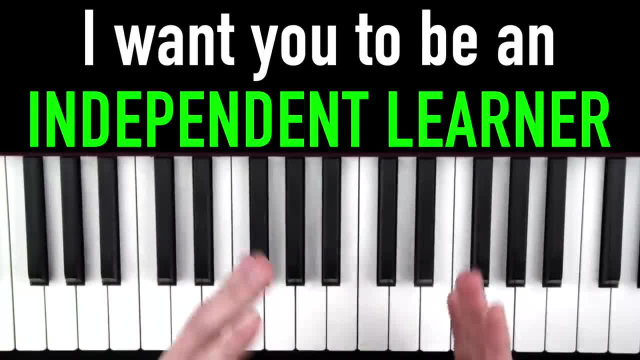 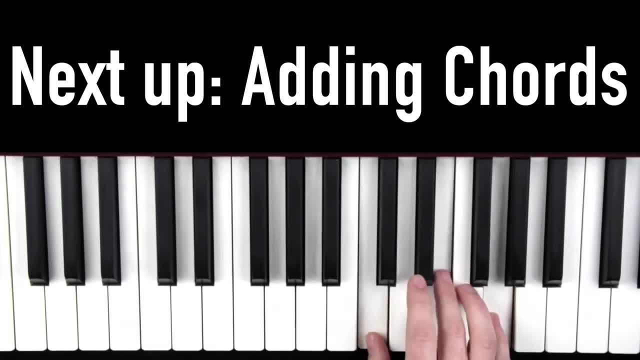 but I'm actually showing you the process of how to learn for yourself, step by step. That way, you can learn anything you want on piano. Alright, so next up, we're going to start adding in different chords to make these rhythms actually sound like they would in a song. 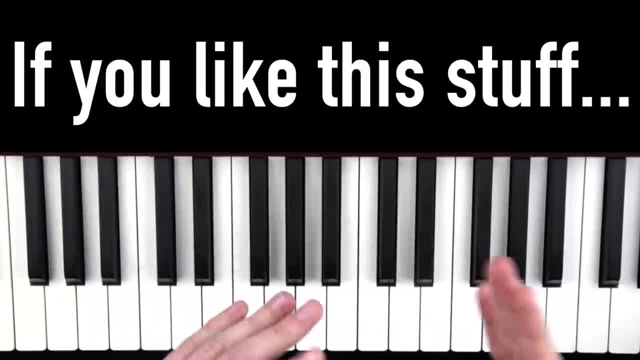 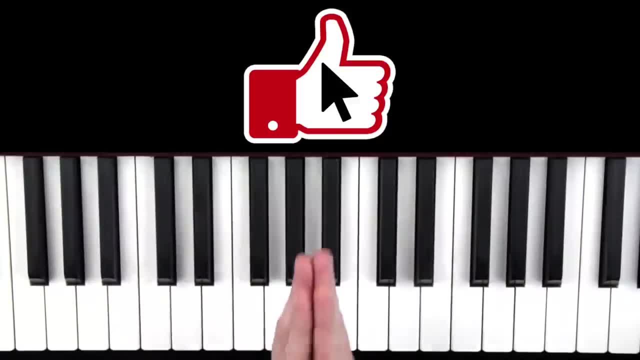 But first, if you like this style of teaching where I really take baby steps and teach you not just what to do but also the process of how to learn, if you could hit that like button, I would really appreciate it. Thank you so much. 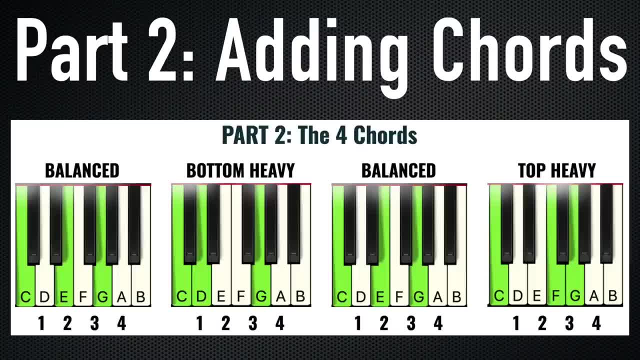 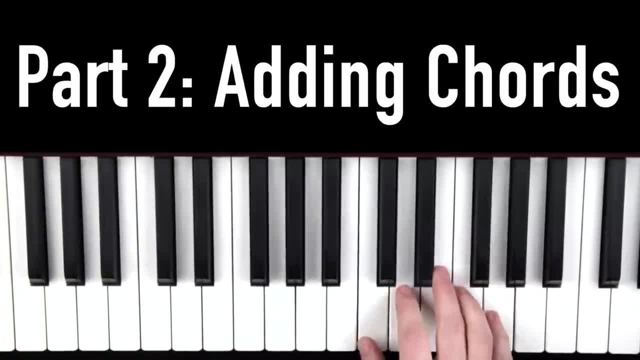 Alright. on to part two, adding chords. Alright, so next up, instead of just playing these three notes, we're going to practice rhythms over the top of different chords. Now, if you're already advanced, you can take any chords and just play a rhythm over it. 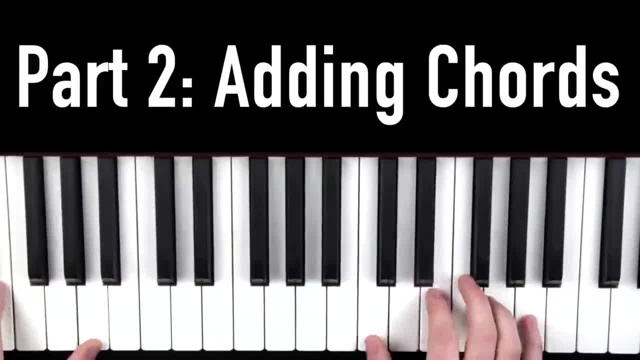 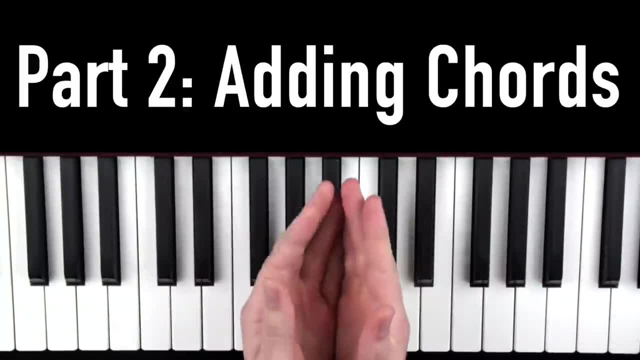 And you can just say, okay, C major, G major, A minor, F major. But if you're a beginner, we're going to simplify it tremendously, but it is still going to sound good. Alright, so our first chord is actually really easy. 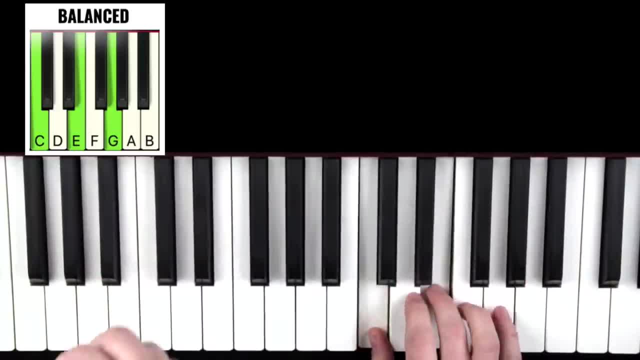 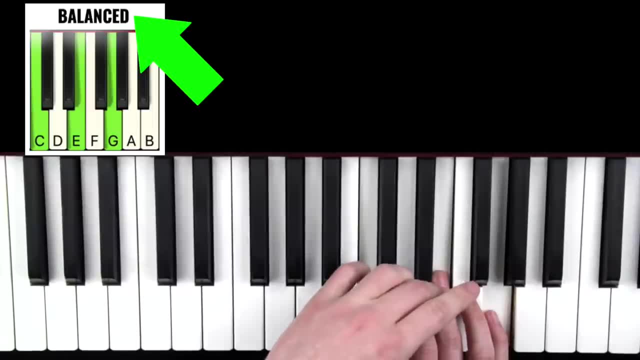 It's actually the chord. we already learned Our C, E and G And just for this video, we're going to call this chord balanced right. Because, just to make it easier for you, because it's balanced right. 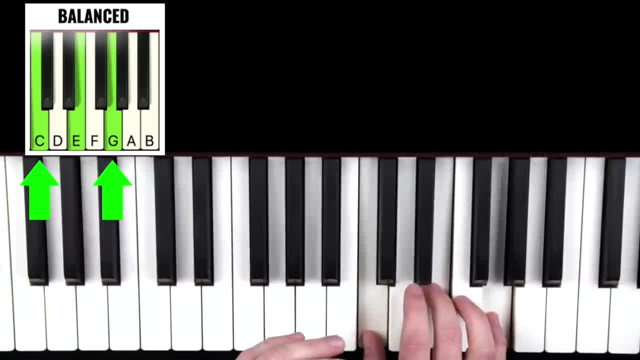 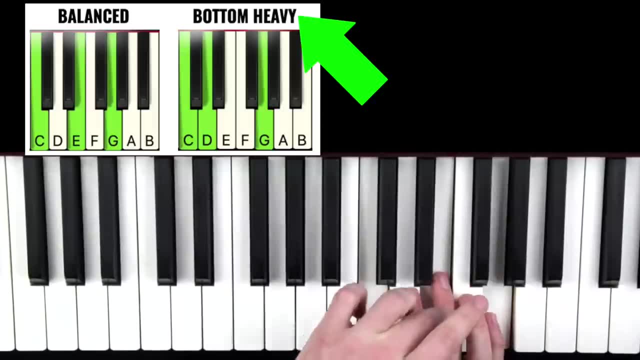 The middle note is right in the middle of these outside notes. Now for our second chord. we're going to call this chord bottom heavy, okay, And the only thing that changes is we're going to take this middle note E. 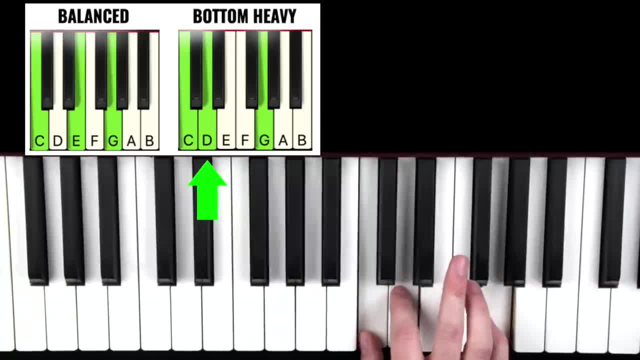 and move it down to your second finger playing D, So you notice the outsides. your thumb and your pinky stay completely the same. They don't change at all. You just change the middle note from an E down to a D. 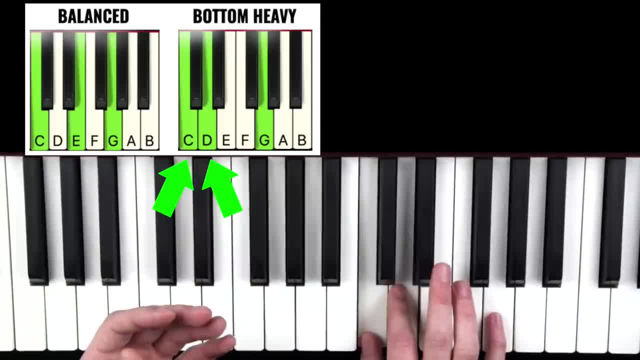 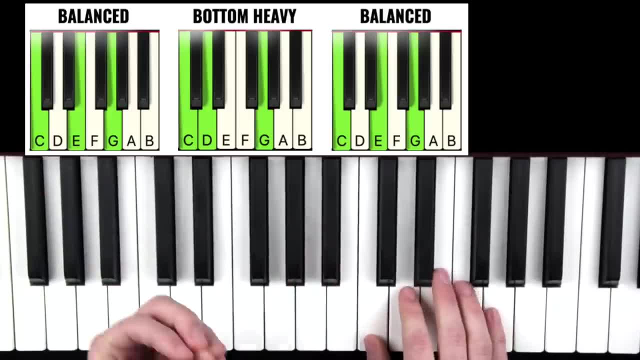 That's it, And we call it bottom heavy, because there are two notes on bottom and only one note on top. And then for our third chord, it's easy: We just go right back to our balanced chord. So so far we have balanced. 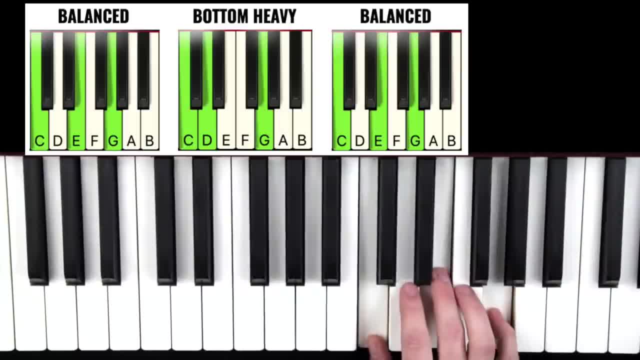 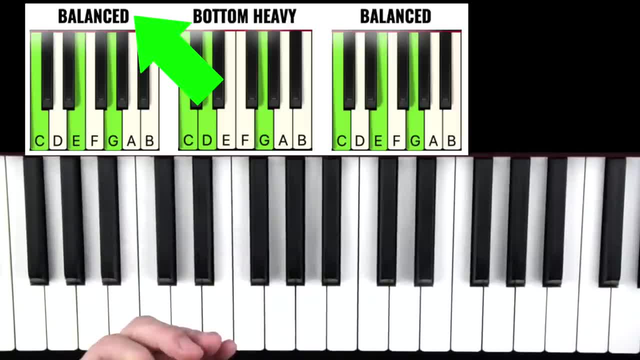 then we go down to bottom heavy and then to balanced. Those are our three chords so far. So right now I want you to practice for a bit just going back and forth between balanced and bottom heavy. So just practice alternating balanced, bottom heavy. 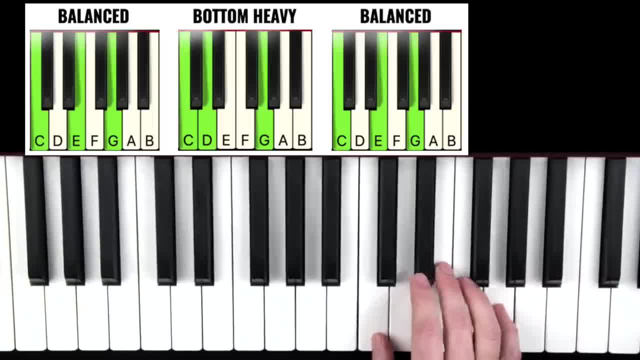 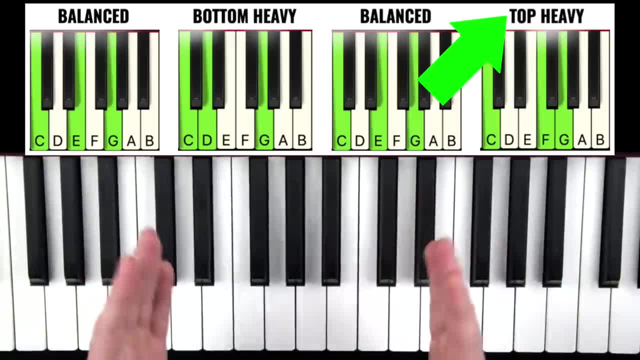 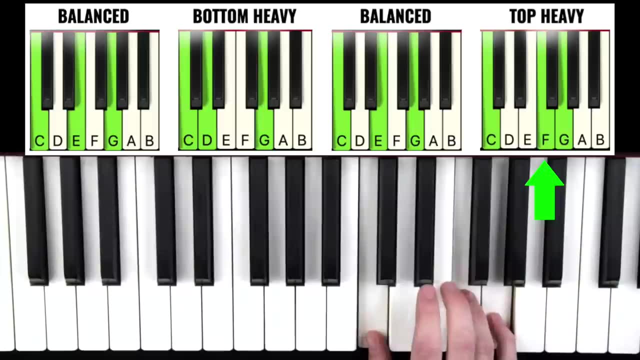 balanced, bottom heavy and really just drill this into your bones. Now for our fourth and final chord. this is going to be called top heavy and it's exactly like balanced, except instead of this E, we're going to move it up to our fourth finger playing F. 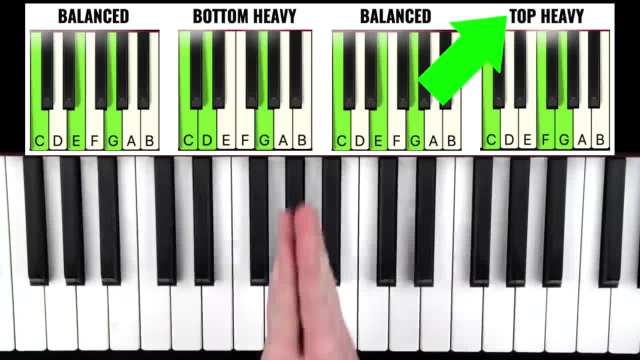 So it's going to look like this, And I'm going to call this chord top heavy, because it has two notes on top and only one on the bottom. So now practice going back and forth between balanced top heavy, balanced top heavy. 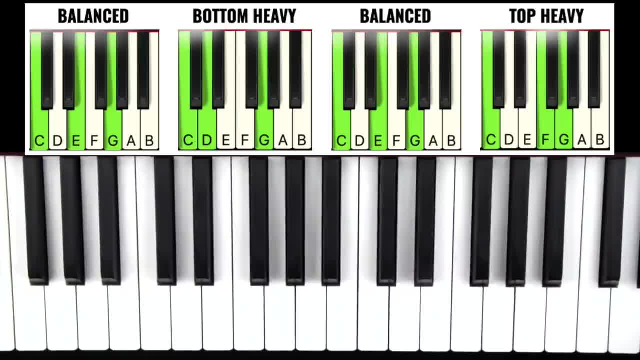 and just really drill this into your bones, Alright, so once you have that, good, let's put it all together. So the whole chord progression is going to go: balanced bottom heavy, balanced top heavy And, we repeat, Balanced bottom heavy. 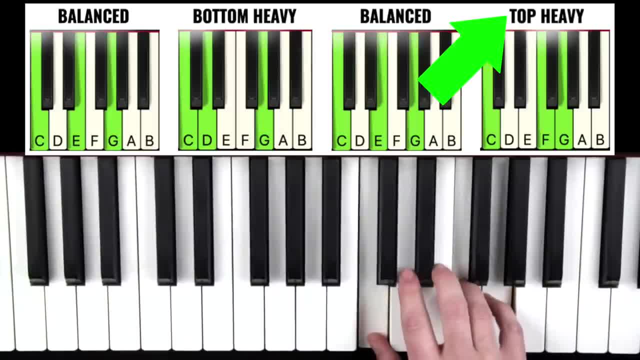 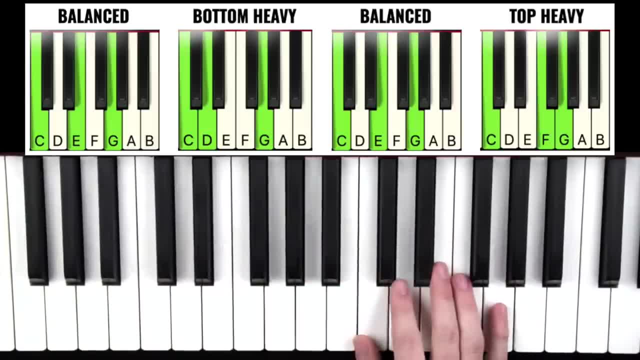 balanced, top heavy. So practice those four chords for a bit. Really, get it into your fingers. And once you have it good, we're going to start adding the rhythms over the top of this chord progression. And this is when it really starts to get fun. 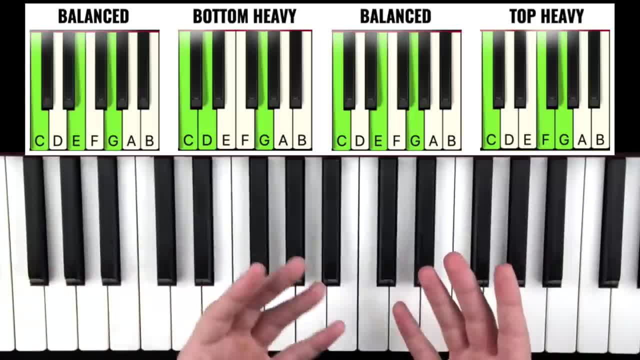 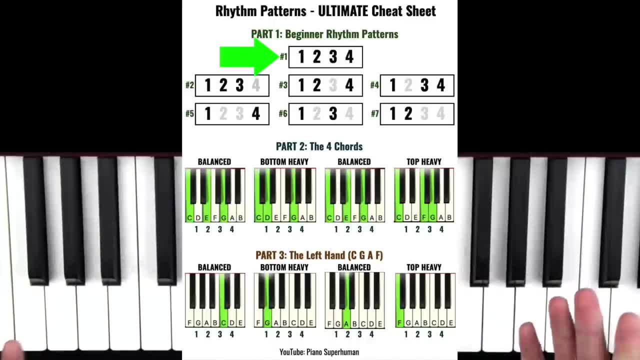 and it really sounds like how chords actually sound in an actual song. So let's go to the cheat sheet and find beginner rhythm number one. So this is the simple rhythm: One, two, three, four. Now we're going to just put it over the chords. 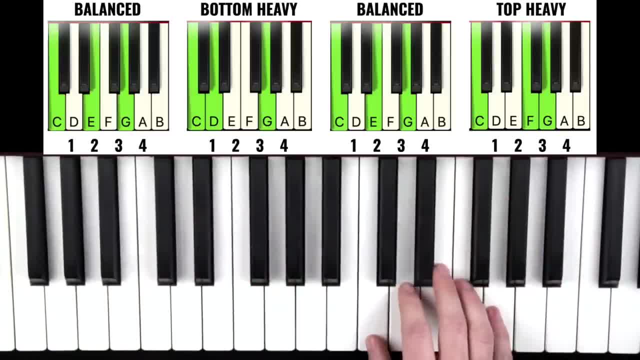 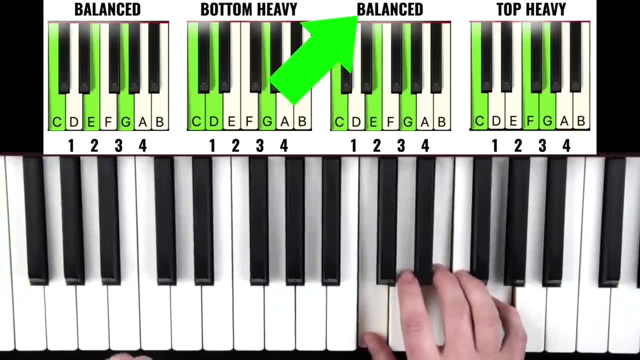 So it's going to sound like this: We're going to start with our balanced chord: One, two, three, four. Bottom heavy. One, two, three, four. Balanced One, two, three, four. Top heavy. 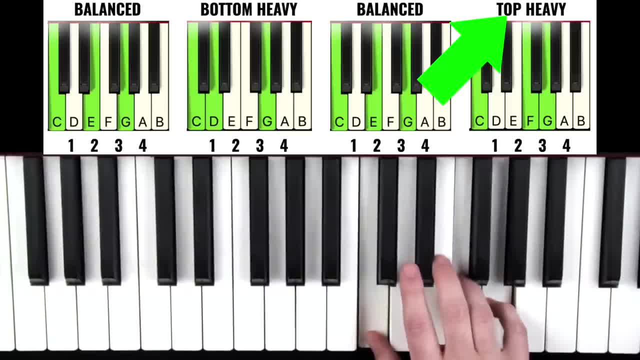 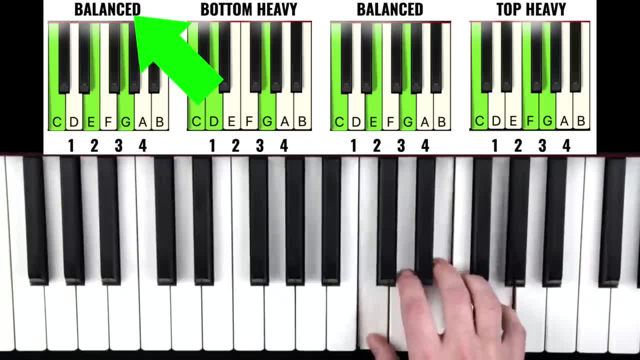 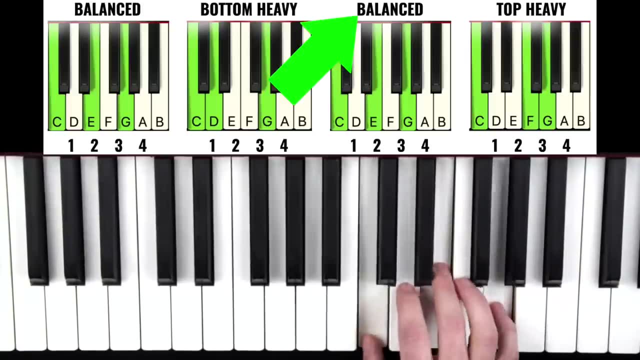 One, two, three, four, And we can repeat: Balanced One, two, three, four. Bottom heavy: One, two, three, four. Balanced One, two, three, four. Top heavy: One, two. 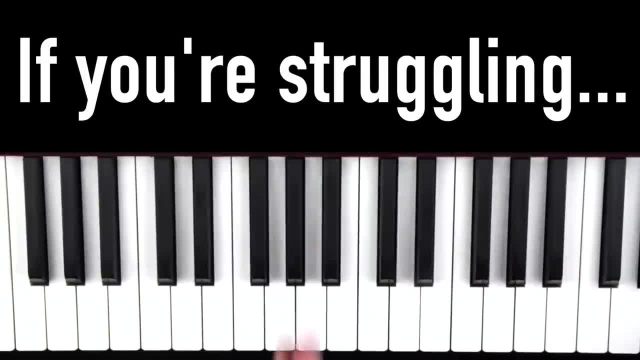 three, four. Now this step is the toughest part for beginners, So if you're struggling here, don't worry. There are three things you can do if you're really having trouble with this step. Number one: slow down. Most beginners make the mistake of trying to play this way too fast. 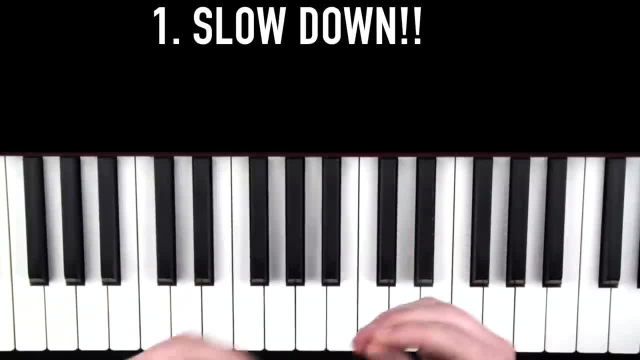 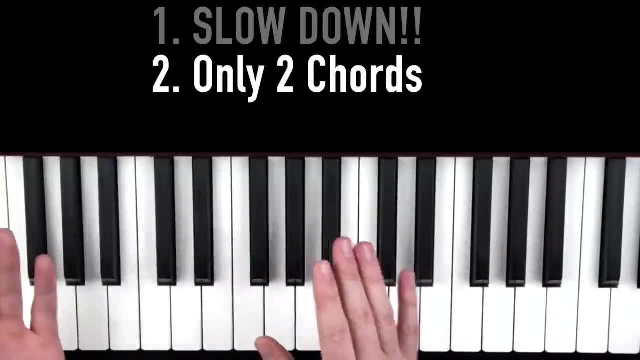 You can always add in speed later, But it's better to have it slow and accurate. first Number two: you can try practicing just two chords at once, So we can just practice going from balanced to bottom, heavy over and over, like this Balanced. 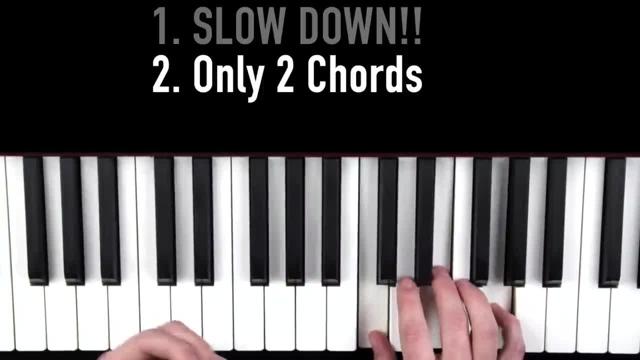 Two, three, four. Bottom heavy. One, two, three, four, Balanced One, two, three, four. Bottom heavy. One, two, three, four, And you can do the same thing with balanced to top heavy and then, once you have that, good. 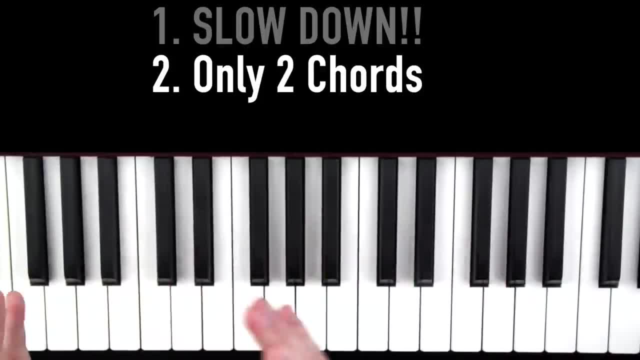 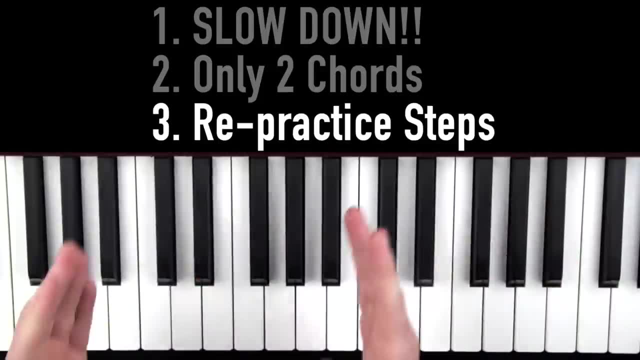 you can add them together. So we're basically taking smaller sections, learning them and then putting them back together. And number three: if you're still struggling with this, go back and redo the easier exercises earlier in this video. Really drill it into your fingers and then come back to this afterwards. 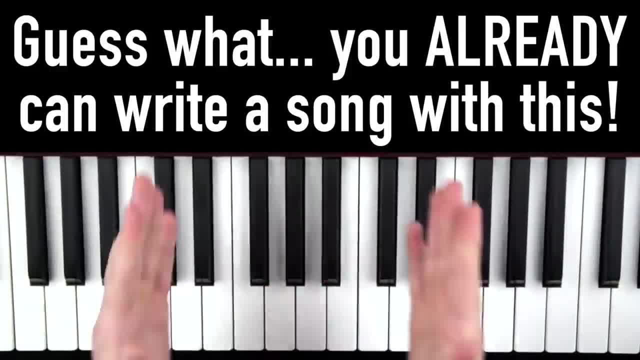 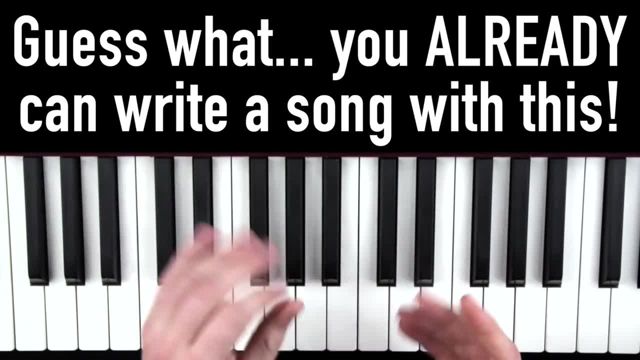 Now check this out. At this point in the video I didn't tell you yet, but you already actually have a pattern that you could literally write a song to, even before we add the left hand. Alright, so once you practice this a bit and speed it up. 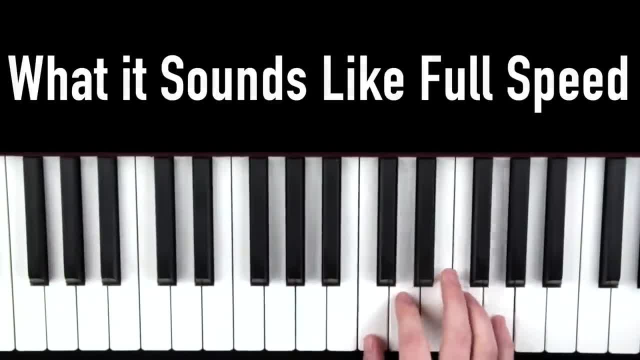 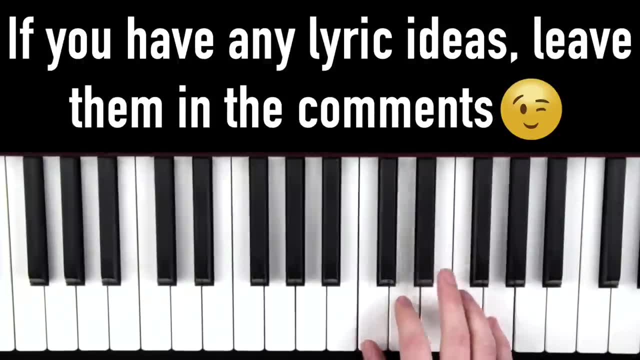 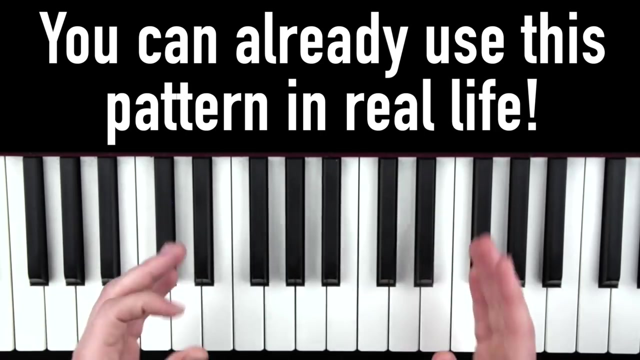 it's going to sound like this And you can actually sing along to it right Now. obviously, I'm not a singer, I'm not actually good at singing, but if you had a good singer or you could actually sing, you're already good, right. 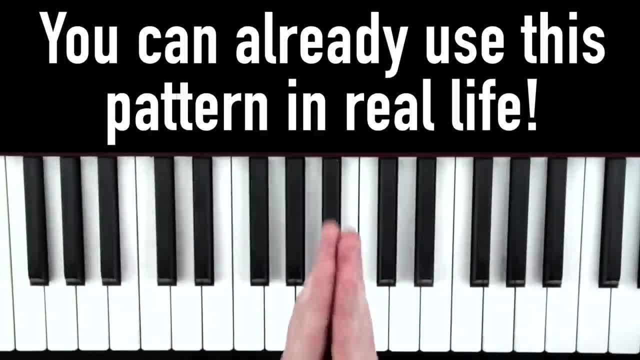 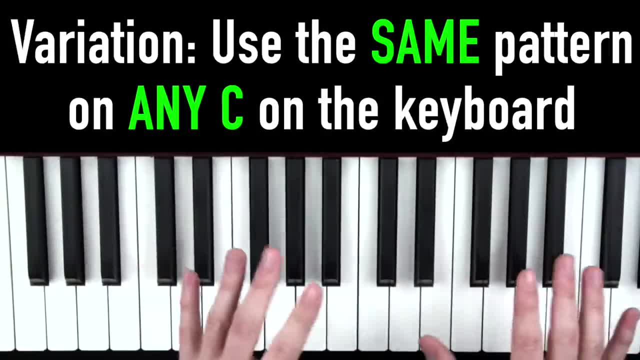 You already have a chord progression that you could write a song with, and it sounds good with this pattern, even before we add the left hand. What's even cooler is- I didn't tell you this yet, but you can take this pattern and you can move it to any C on the keyboard. 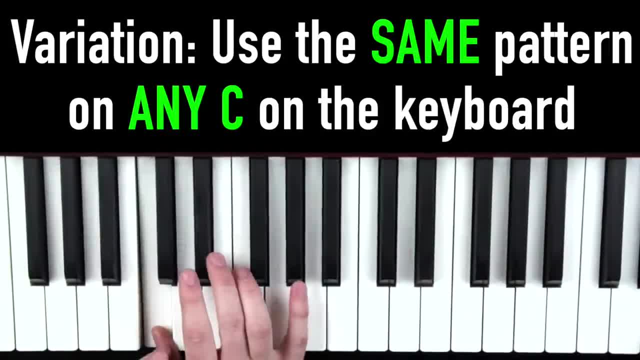 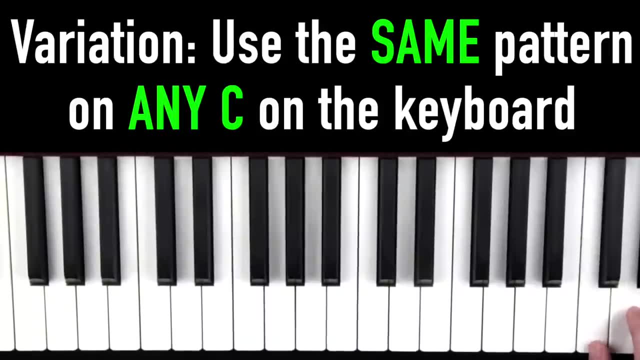 So find any two black notes, play your thumb on C, and this pattern will always sound good. So you can play it here Or up here, And it's always going to sound good. So now, even though you learned this one pattern, 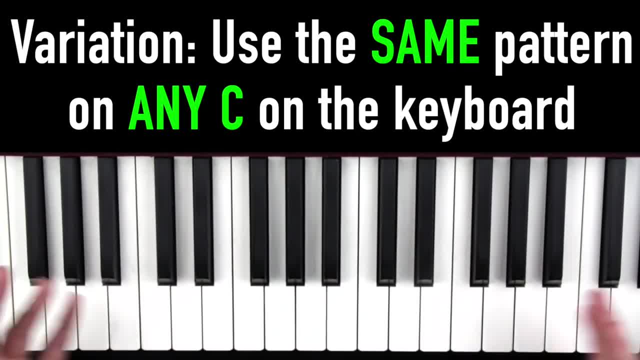 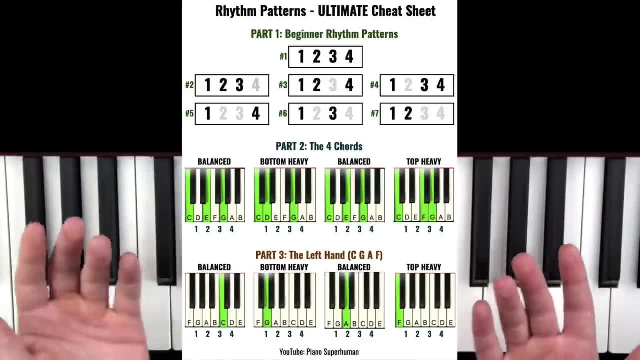 you actually have a lot of different options already that you can use up and down the keyboard, And of course we can do this with any pattern on the cheat sheet. So that was just with pattern number one. one, two, three, four. 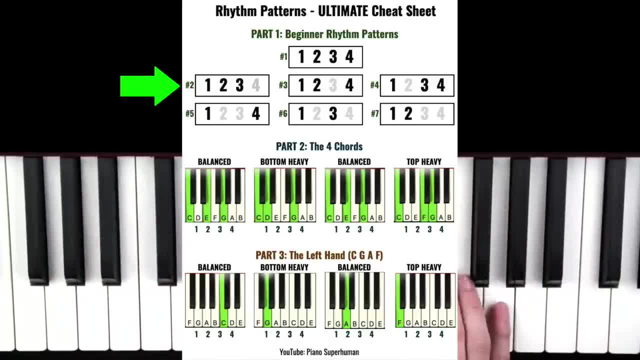 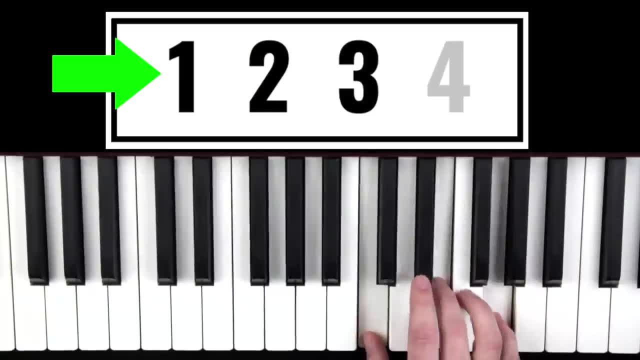 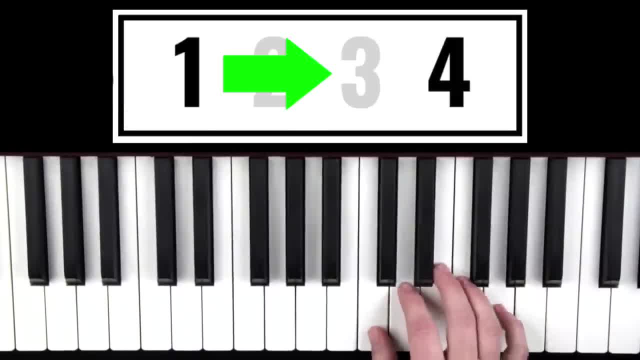 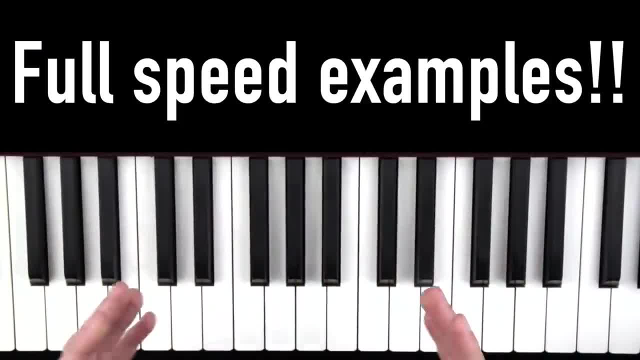 and it's always going to sound good. Alright, so let me just show you what a few of these are going to sound like, What they're going to sound like at full speed, And I'll add in the left hand, just so you can hear. 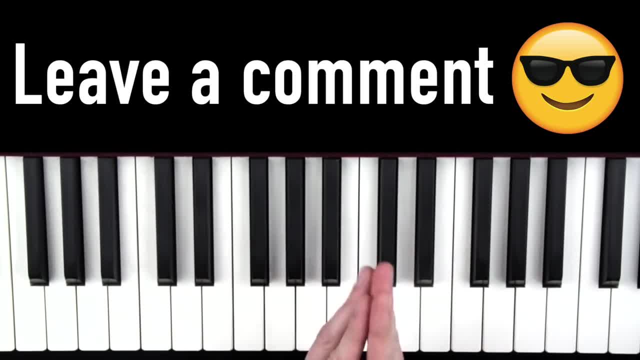 kind of what the final product sounds like, And I'm going to show you the left hand in a bit, Alright, so let me know in the comments which one of these is your favorite, Alright, so here's what rhythm number three sounds like at full speed. 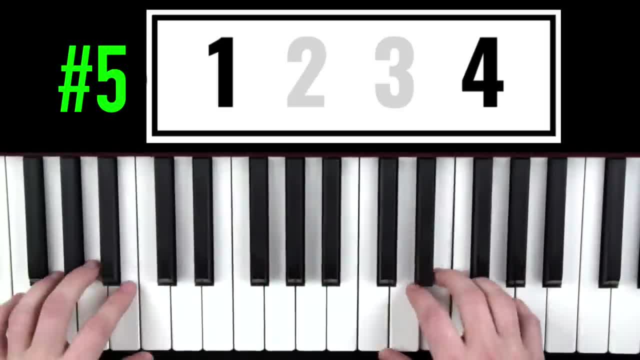 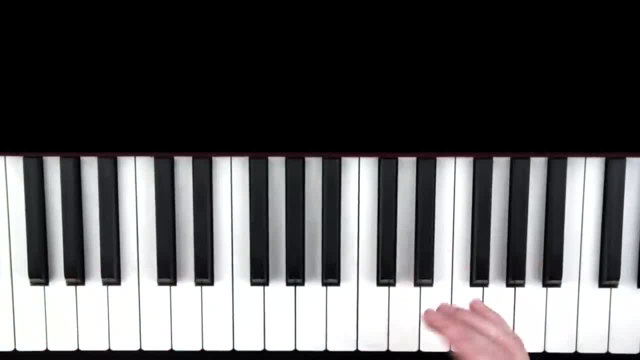 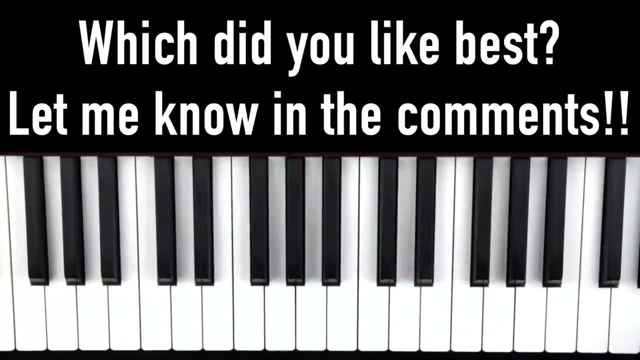 Here's what rhythm five sounds like at full speed And rhythm number seven at full speed. So I'm curious which of those did you like best: Rhythm three, rhythm five or rhythm number seven? Let me know in the comments. 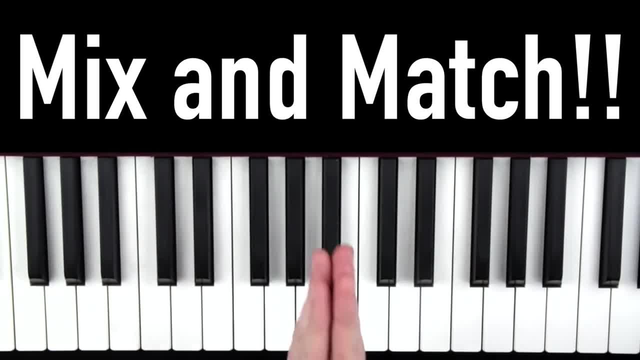 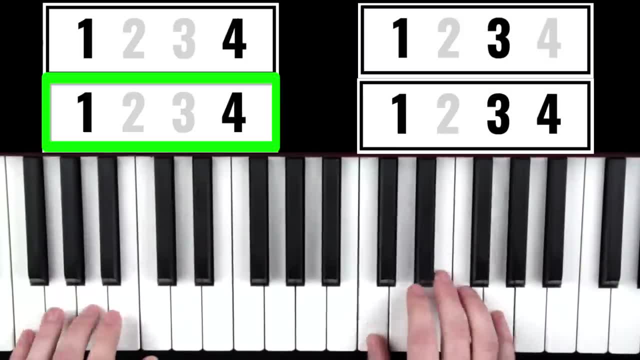 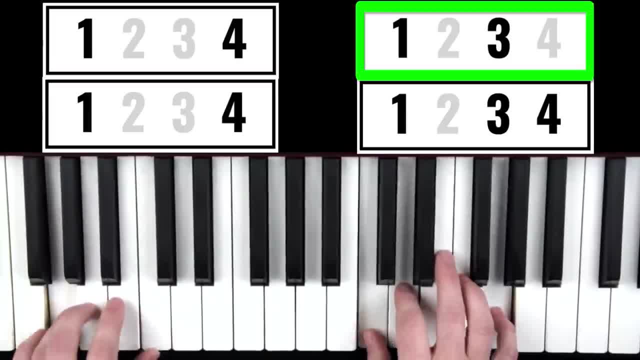 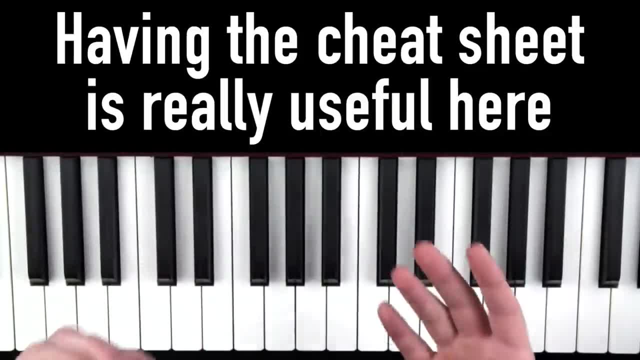 One, two, three, four. One, two, three, four. So be creative, Come up with your own combinations of patterns. This is where having the cheat sheet really comes in handy. Alright, so next up, we have adding in the left hand. 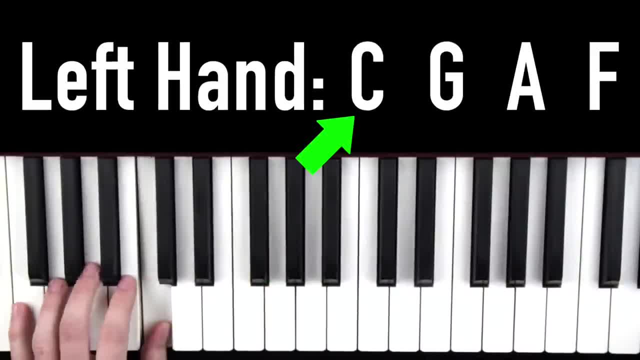 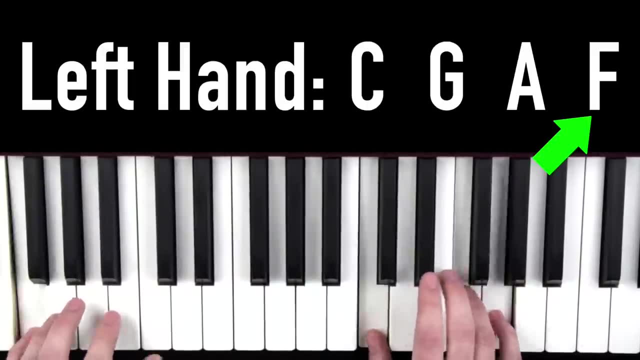 Now the short and simple version is: the left hand simply plays C, then G, then A, then F. So if we play it along with the right hand, it's going to sound like this: G A, F. Now this video is getting a little bit long. 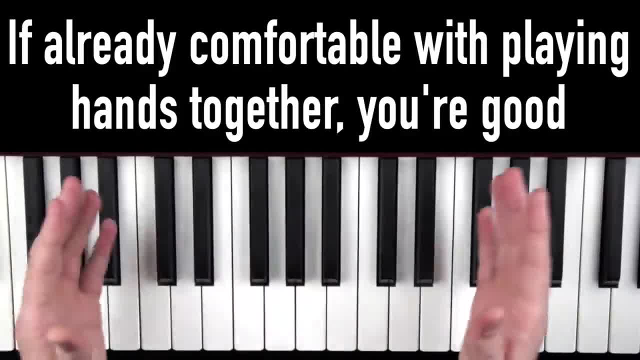 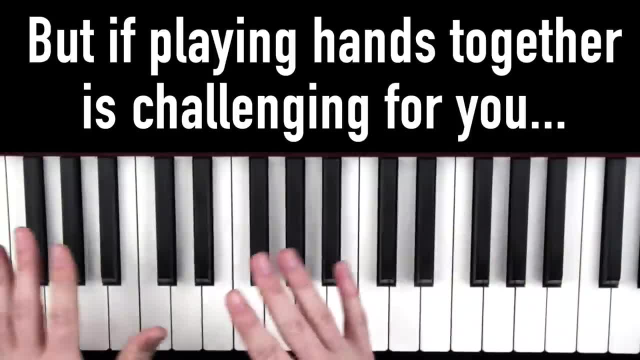 so if you're already good at getting hands together, you can just learn it right here and you're good. But if you're not, and you really want the down and dirty, step-by-step process to learning the left hand, just like we learned everything else in this video, 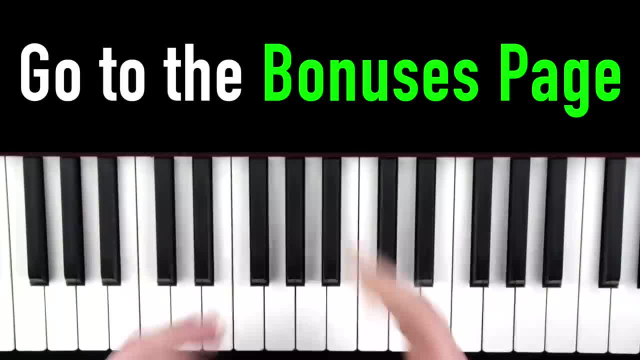 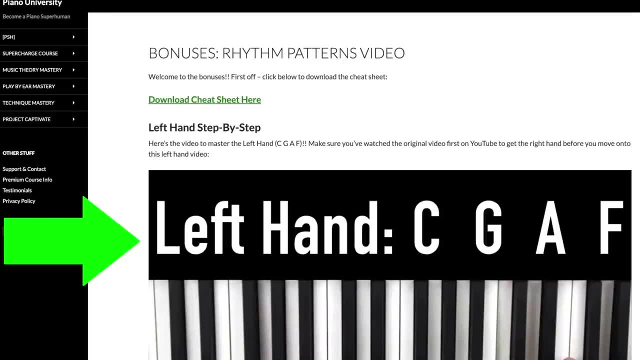 by taking very small baby steps to make sure that you don't get frustrated. if you go to the bonuses page, which is the exact same page you downloaded the cheat sheet, underneath the cheat sheet you can go to the left hand instructions video and I'll break it down step-by-step. 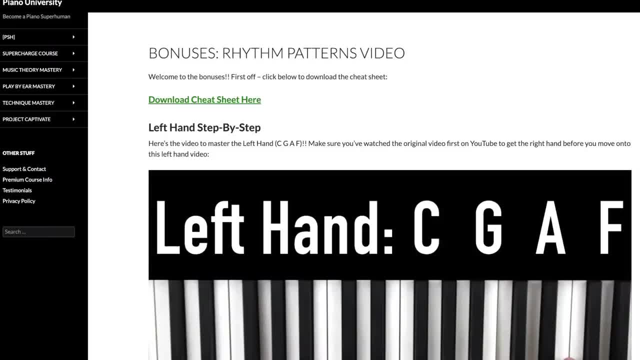 So click the link, if you haven't already put in your name and email, and go get your bonuses now. And then I'm also going to have part two of this series coming out soon, which is going to have intermediate and advanced rhythm patterns. 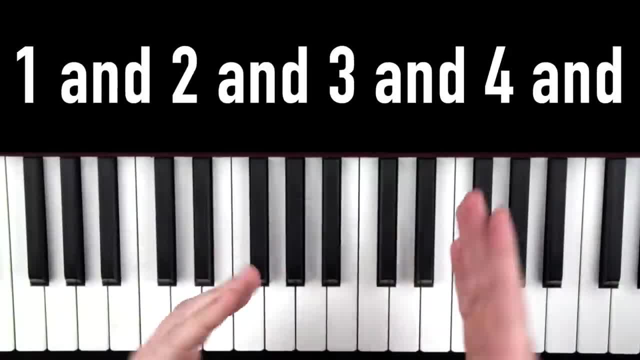 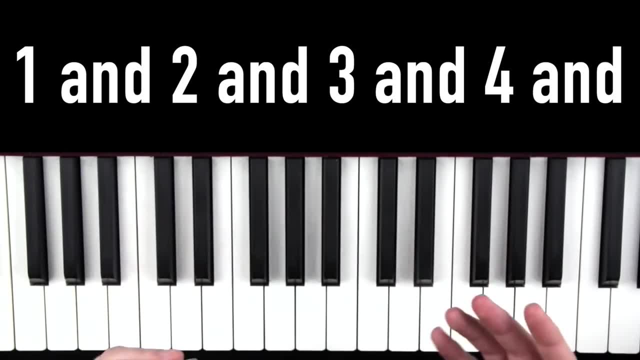 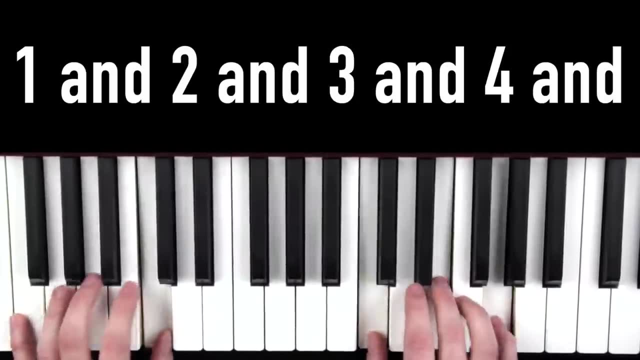 which are a bit faster, And if you've ever heard somebody count one and two and three and four, and this is what they're using and it allows you to play more complex stuff like this. If you want more of this stuff, be on the lookout for part two.